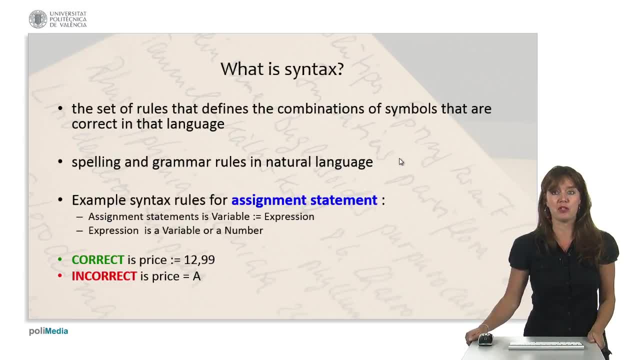 which is an assignment statement. Assignment statements are used very often in programming. So here you see that an assignment statement is a variable, a colon, an equal sign and then an expression. So it's composed of three parts: A variable, a colon and equal sign together and an expression. 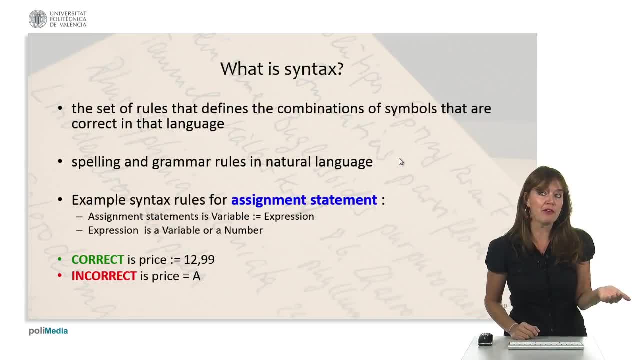 And an expression can then be, for example, another variable or a number. So if this is the rule for writing down assignment statements, you can see that here in the green one the correct assignment statement is this: one Price, a colon, an equal sign and a number. 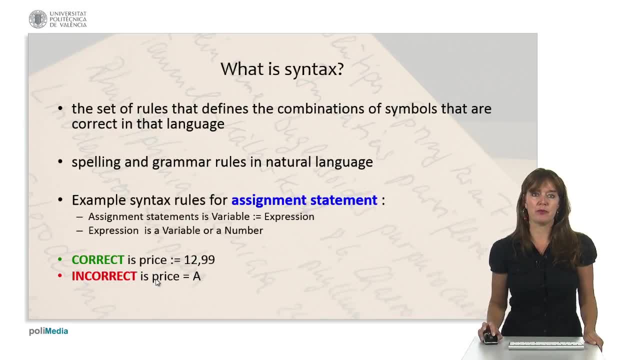 An incorrect assignment statement. you see here below, with the red Price is a variable, but this is wrong because it's only an equal sign and the colon is missing And, moreover, this is an A, which is not a number. So this is a syntax rule indicating how we have to write down assignment statements. 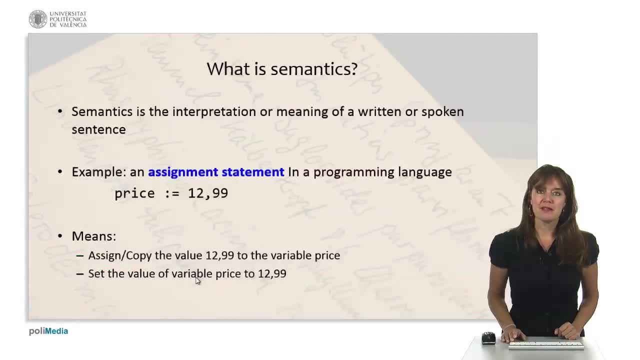 So this is syntax. What is semantics? Semantics is the meaning or interpretation of all the statements that you can write. So we have seen how we can compose an assignment statement correctly. Now we look at what it means. What it means to say that we want to do price colon equal sign 12.99.. 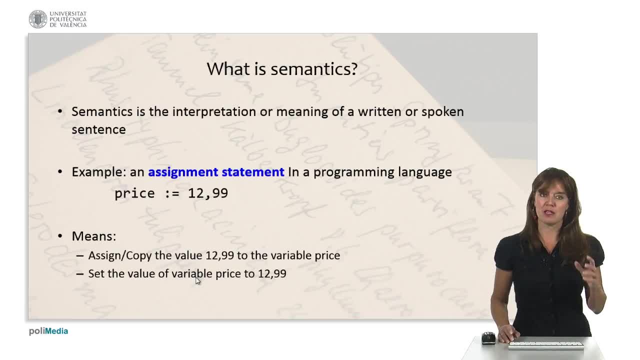 What does that mean? Syntactically it's correct. Semantically it means assign or copy the value 12.99 into the variable price. Or another way to say it set the value of variable price to the number 12.99.. 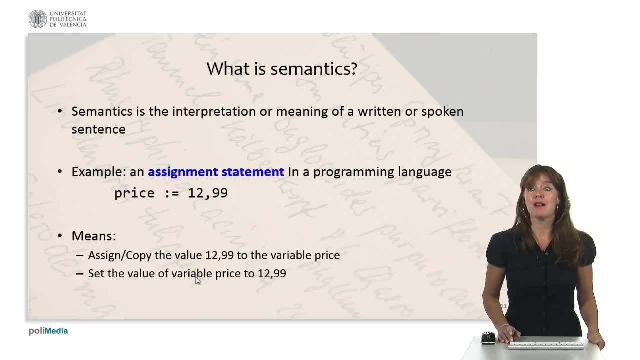 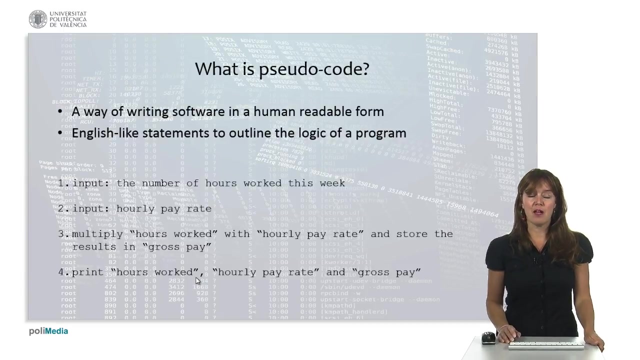 Or if you are a programmer, you would say: assign the number 12.99 to the variable price. So syntax is how you have to write statements that are correct. Semantics indicates what they mean. So, finally, a concept we want to see because we are going to use this in the other parts.